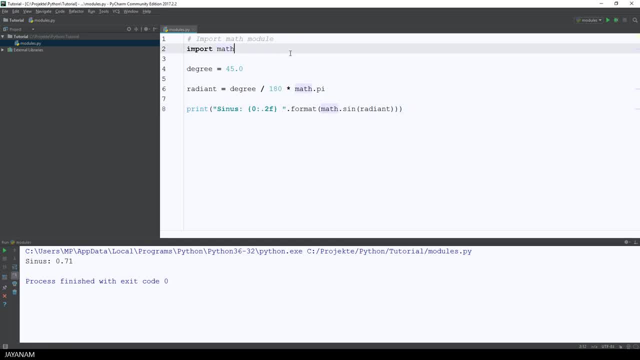 All right, you can also go ahead and just import the sine function and the pi definition and not the whole module. To do this, you write from then the name of the module, followed by the functions you want to import. In our case, this is from math: import sine comma, pi. And now you call these functions as: 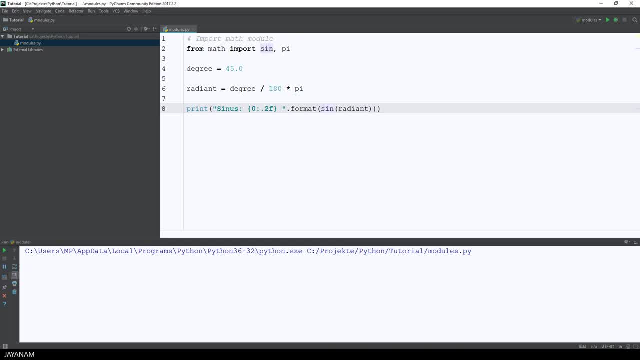 if they were defined in the current file without the module's name as prefix. Another option for importing modules is to define an alias For the imported module. then you write import, then the name of the module s, followed by the alias. Here I defined m as alias for the math module, So I have to use m as prefix to call the. 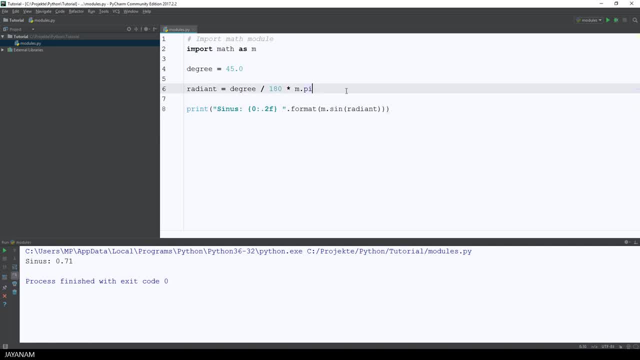 functions of the math module. Okay, what I'm going to do now is to define a function called get sine that calculates the sine value for a degree parameter. I'm adding this because I want to use the radians as a value in the. I want to treat my modulespy file as a custom module that I will import into a file that I'm going to create later on. 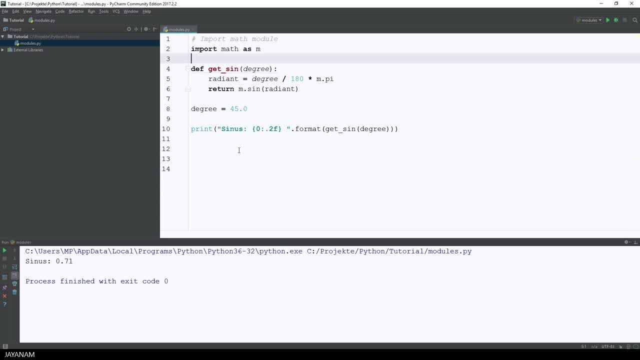 After importing this, I will have access to the function getSign that I just created. So let's do this. Let's add a new Python file to the project and call it module test. So here's the empty file, And now let's import the modules file as module, just like we did before for the math module. 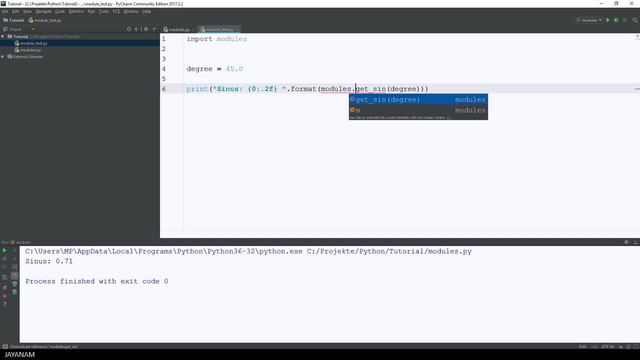 And now we are able to call the getSign function from our own custom module. Of course, you can also just import the getSign function. Then you write from modules: import getSign. The last thing that I want to show you is using the package manager PIP. 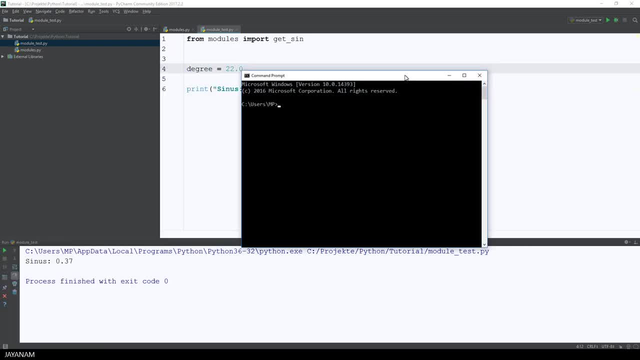 that comes with Python. To install external packages, Just open the command prompt and type in PIP install and then the name of the package, like numpy, here Think of packages as collections of modules, and numpy is a fundamental package for scientific computing with Python.